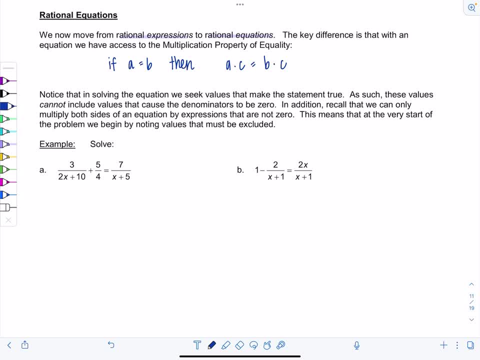 values that make the statement true. right, An equation is a statement As such. these values cannot include values that cause the denominators to be zero, So this is going to be something we will address at the very beginning, before we start solving any equation. In addition, recall that we 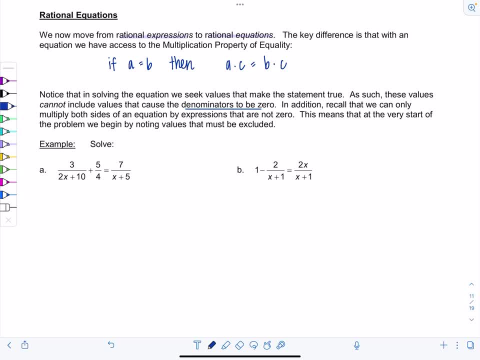 can only multiply both sides of an equation by expressions that are not zero. So this means that at the very start of the problem, we begin by noting values that must be excluded, listing the restrictions, basically. okay, So basically your steps to solve are going to be that you want. 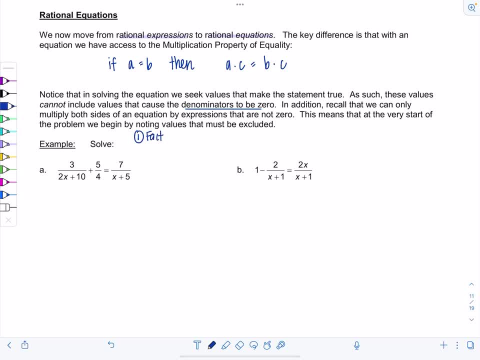 to factor all your denominators. You want to list your restrictions And then you want to multiply both sides of the equation by the LCD to make your equation fraction-free. okay, So there should be no more denominators after you complete step 3.. If there, 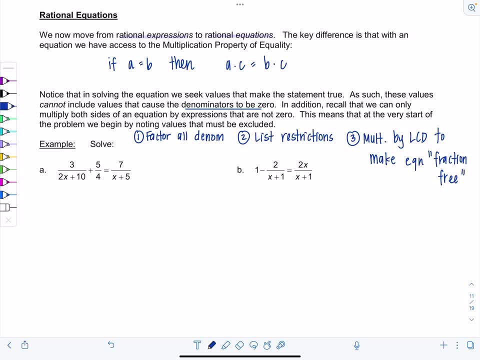 are you messed up somewhere? okay, Then you solve and I say, put your final answer in a solution set. We'll talk about why. But these are just simple steps. So let's start solving. So let's start with the first three steps to get you rolling. okay, Here we go. So example A: solve. We have 3 over. 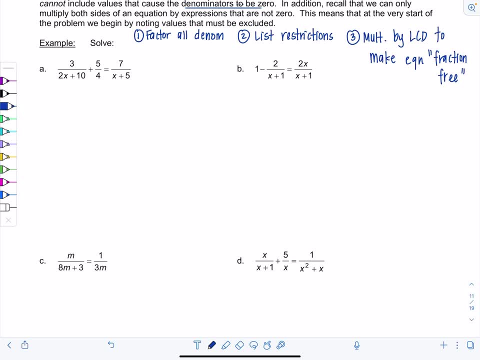 2x plus 10 plus 5 over 4 equals 7 over x plus 5.. So I'm going to start off by factoring all the denominators. Really, there's only one to factor, that first one: 2x plus 10.. So I can take a 2 out. 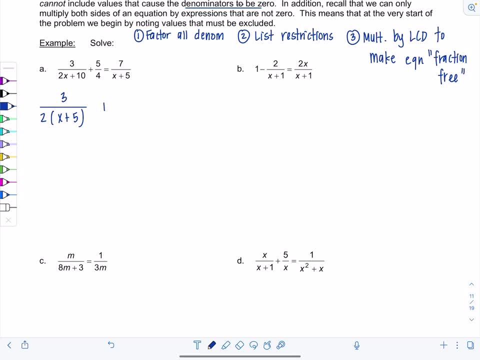 and I have x plus 5 left plus 5 over 4.. So I'm going to start off by factoring all the denominators: 2x plus 10 plus 5 over 4 equals 7 over x plus 5.. All right, So right off the bat, I notice we have. 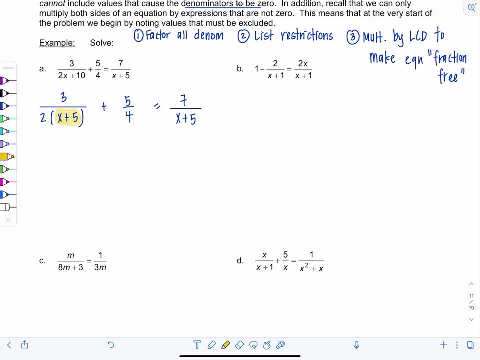 a restriction, x cannot equal negative 5. Otherwise these two denominators would be 0,, which would make the rational expressions undefined. I don't have to worry about the constants 2 and 4. Those aren't changing. That's what it means to be a constant right, Not like. 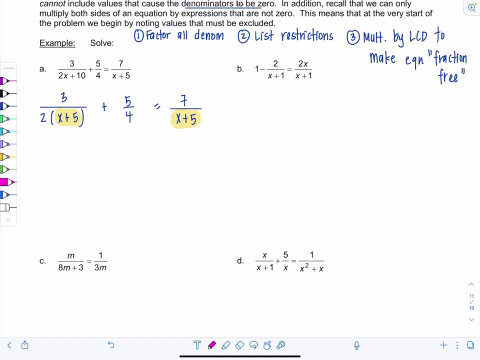 a variable. So those are staying the same. So just remind yourself that you don't have to. x cannot be negative 5.. Okay, Next step is we want to multiply the entire equation by the LCD. So think back a previous lesson, when we were adding and subtracting rational expressions. 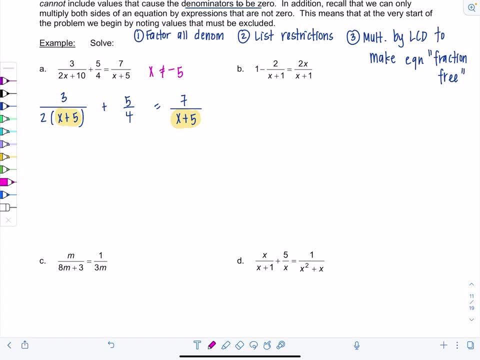 how to find the LCD. So you list every single factor that appears in each of the denominators, but don't repeat any, right? So 2 and x plus 5 need to be in the LCD, But then there's 4. So I need to have a 4 and x plus 5. But like 8 would be too much, right You? 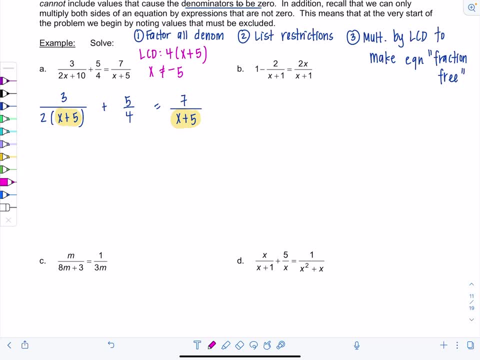 don't need 2 times 4.. So I'm going to multiply everything by 4 and x plus 5.. So this gets hit with a 4 and an x plus 5.. This gets hit with a 4 and an x plus 5.. And same thing over here. 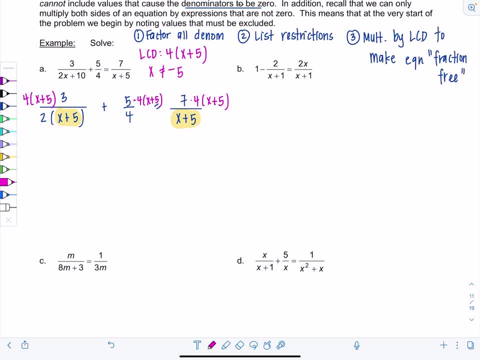 4 and x plus 5.. Always multiply by that LCD. So what's this? This is a 2.. So I have to put this into the numerator. So it's over 1.. So if you need to do a numerator, you have to put the top in the numerator. If you need to remind, 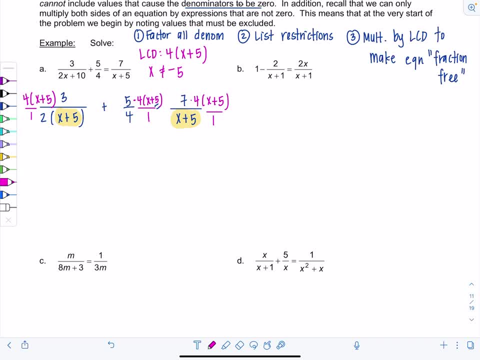 yourself that it's over 1, you can do so. I think it's a little too messy. But the goal is to be fraction-free, Not to get a common denominator, but rather to get rid of the denominators. Okay, So let's see what cancels out. See how x plus 5 is gone. Love it. And then 4 and 2 reduces. 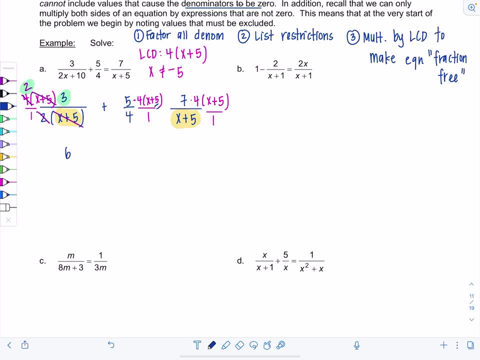 two times three, so that's six. What about the next term? What's canceling out here? So the four cancels, that's it. So what survives is five and x plus five. Okay, five times x plus five equals. and then what cancels out on the right hand side? Let's see x plus five. 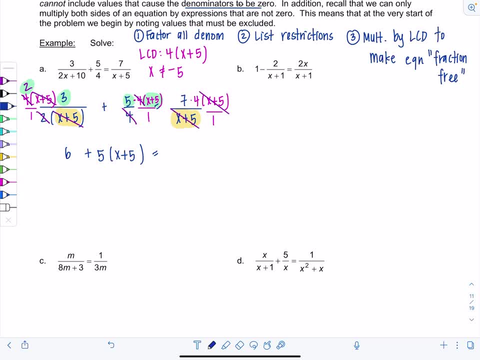 and that's it. So we've got seven times four, that's 28.. All right, looks nice. Now this equation is a lot less threatening, maybe something you remember solving back in beginning algebra, when life was simple. you didn't appreciate it, but it's okay. 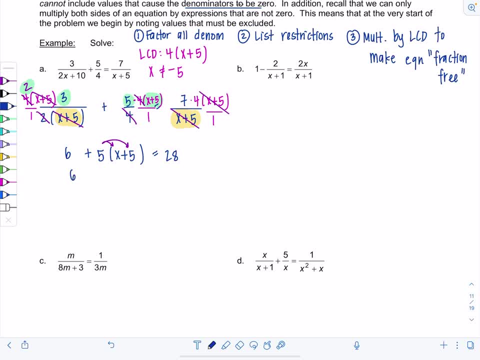 Here we go. distribute that five, So we've got six plus five. x plus 25 equals 28.. I'm gonna keep that five x On the left. six plus 25, that's 31,. 28 minus 31 is negative three. so we got x equals negative three over five. Now 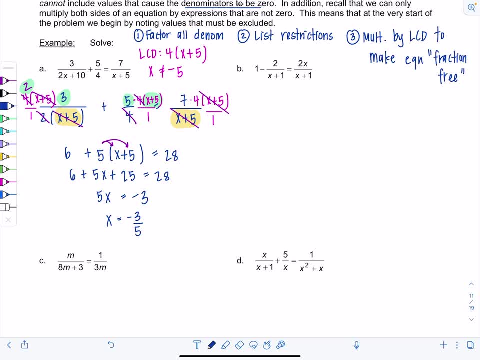 I'm gonna check what was my restriction. x couldn't equal negative five. We're good, so I'm gonna list negative three-fifths now in my solution set as my final answer. Okay, that's the proper way to do it. Your instructor may not recall. let's skip, We can make it a little. upset this time. But which one is x? How does that make it? Okay, let's copy and paste, Alright. So this is a little summary right here. Which one is x equals negative three-fifth. Okay, what was x? why is x wrong? Well, the answer we have here is negative five. 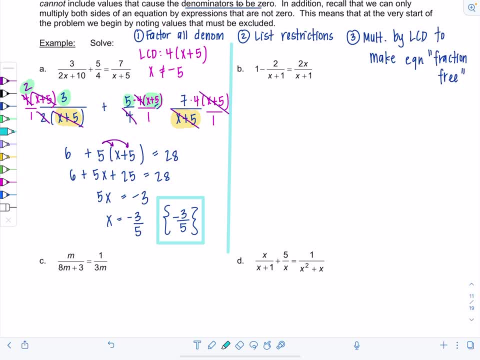 So what startups have to do is multiply five и producing seven до нового require you to do a solution set, but you're going to see why they're beneficial in just a few more examples. okay, Good, So let's look at example B here. 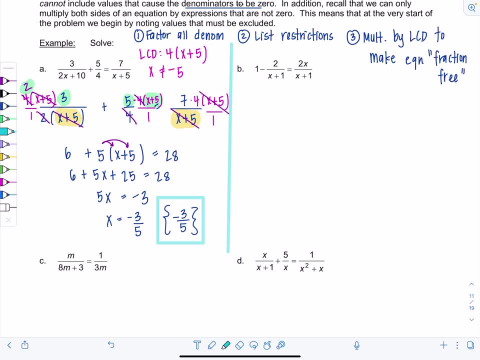 We have 1 minus 2 over x plus 1 equals 2x over x plus 1.. So step one: factor all the denominators. that's done. Step two: list the restrictions. So what do you notice? x cannot be equal to. 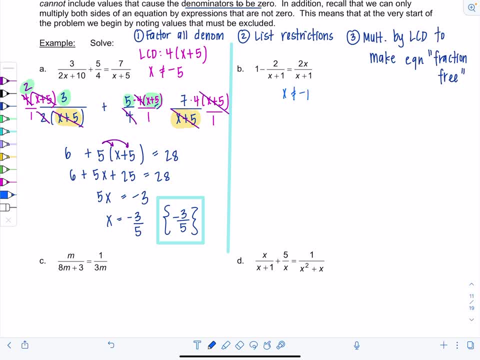 Very good, just negative 1, right x cannot equal negative 1.. And then now let's figure out what the LCD is and multiply the entire equation by it so we can get rid of the denominator. So let me write it more. spread out here: 1 minus 2 over x plus 1 equals 2x over x plus 1.. So what's the LCD? 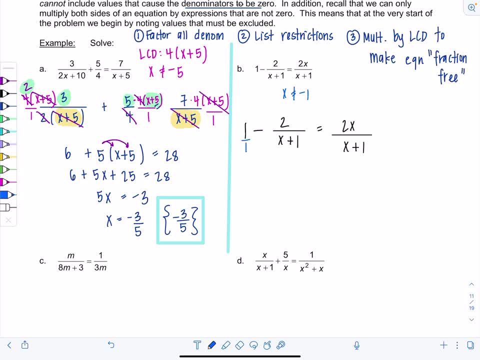 If you want to remind yourself, remember this, 1 is just over 1.. So the LCD is just x plus 1, right, Good. So multiply everything in the equation by x plus 1.. This is the beauty of the multiplication property of equality: Multiply in the top. 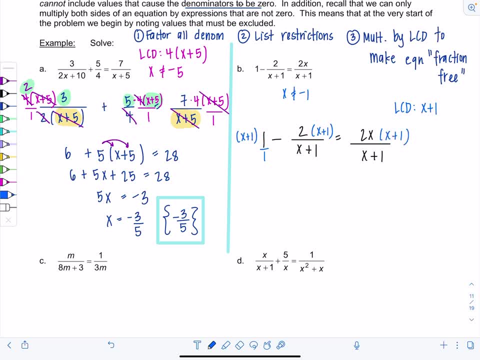 in the numerators. okay, And let's see what we have So right here. in this first term, nothing canceled out, So we're just left with x plus 1, minus notice here that x plus 1 cancels out, So I'm just left with 2. 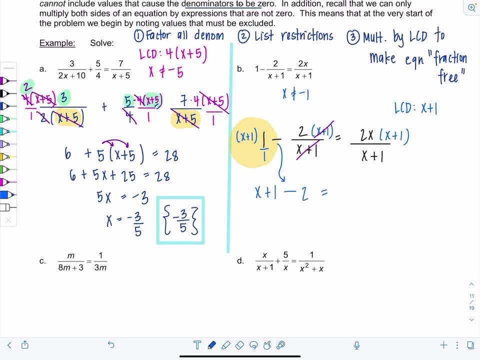 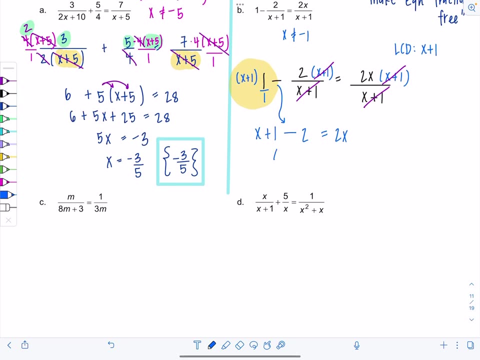 equals. and then same thing over here on the right-hand side of the equation: x plus 1 cancels out, So I have 2x. Okay, so let's clean up on the left-hand side Now. we're going to have x minus 1 equals 2x If I subtract x from both sides. 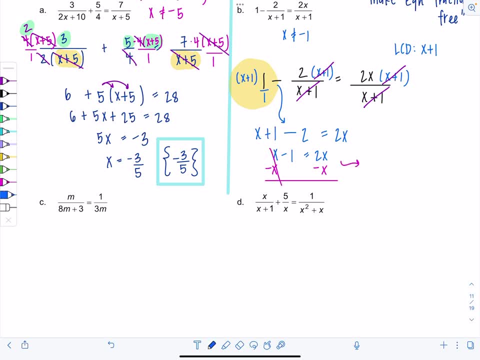 x will cancel out here and then I get negative. 1 is equal to x, But you guys be careful. Wasn't my restriction precisely that that x could not be negative 1?? So that means we cannot report this as our final solution. 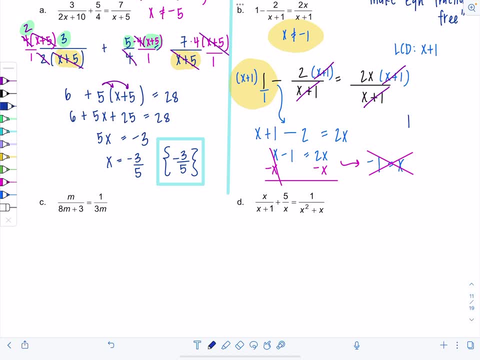 So in fact, this equation has no solution. I know, Don't be upset, It's not your fault. You could write no solution. You could write a solution set with nothing in it- Ooh, do you like that? Or you could write the symbol for the empty set. 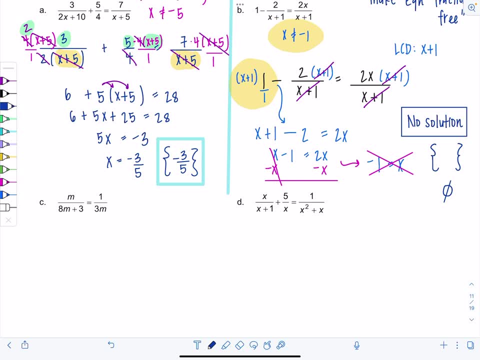 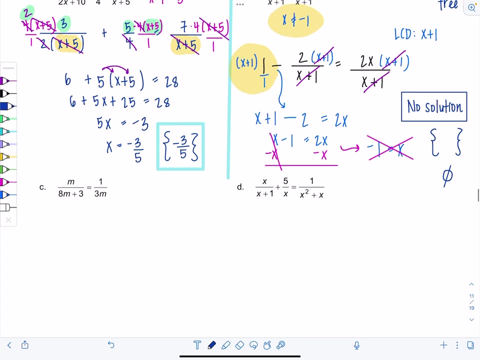 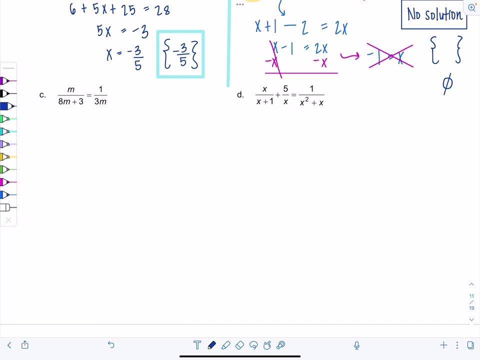 Just don't put that symbol inside your set brackets. okay, That's a no-no. Then it's no longer empty. Boom, All right, Good, good, Let's look at some more. We need some practice here, Okay. Example C: We've got m over 8m plus 3 equals 1 over 3m. 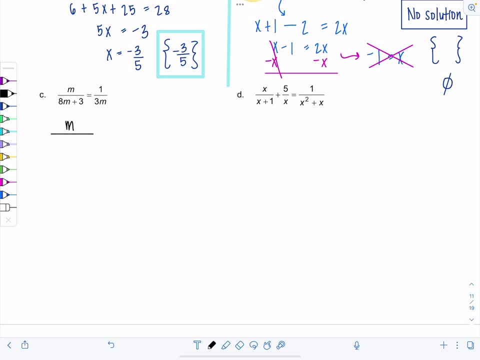 So let me write it out over here: m over 8m plus 3 equals 1 over 3m, So everything's factored. Let's list our restrictions Notice here: 8m plus 3.. We don't want that to be 0.. 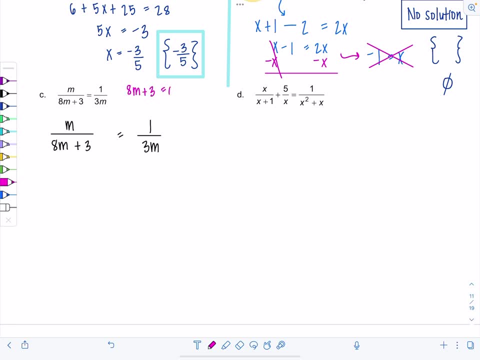 If it's not obvious what the restriction is, just set it equal to 0.. That means 8m equaling negative 3 is a problem, right? These are what we don't want to happen. So m cannot be negative 3 over 8.. 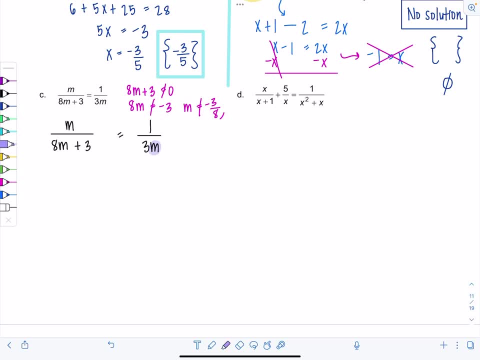 And then when you have just this little lonesome m by itself, not plus or minus anything, then that means m cannot be 0. So these are our restrictions right here. Okay, Now we're going to multiply both sides by the LCD. 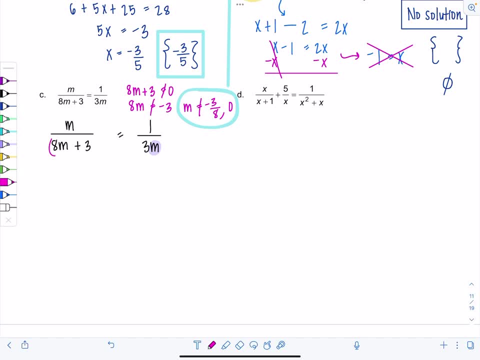 which is basically 8m plus 3 times 3m. You can do that. or in this case, you see how we have one rational expression on the left-hand side and one rational expression on the right-hand side. We can actually cross multiply. 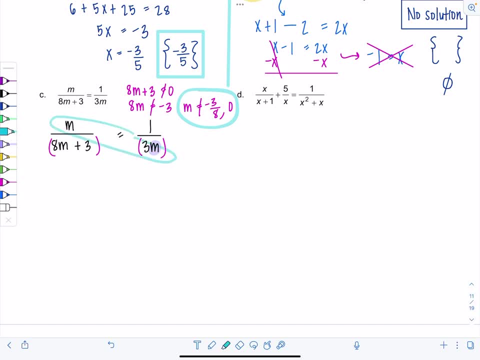 which is a bit easier. Okay, And set those diagonal products equal to each other. So m times 3m that would be 3m squared, And then 8m plus 3 times 1 is 8m plus 3.. 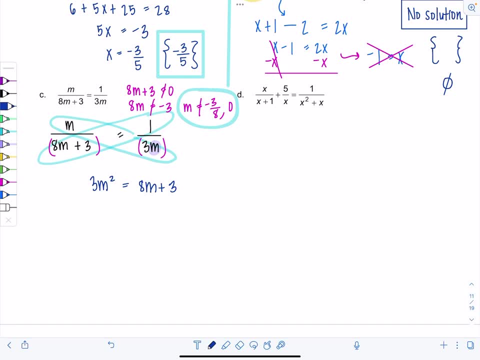 You can only do that when you have one rational expression on each side. Okay, And then from here we have a quadratic equation, So let's set it equal to 0.. 3m squared minus 8m minus 3 equals 0.. 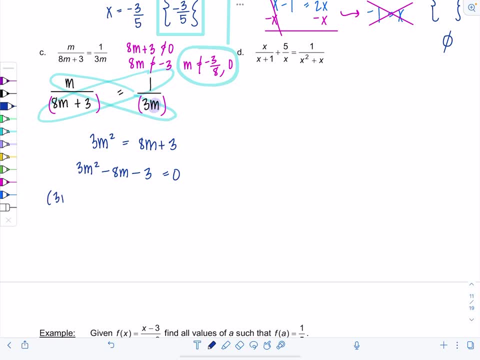 And now we need to factor, So 3m m. If I'm trying to make an 8m in the middle, then I want the 3 here right, So I can get negative 9m with these two guys. 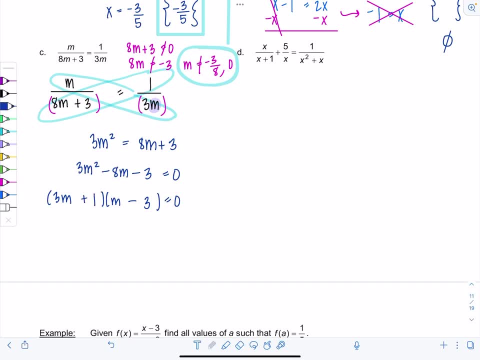 And then a 1 here, and that's going to be positive Yep, And then, using the zero product property, you're going to set each factor equal to 0.. So 3m plus 1 equals 0.. Or m minus 3 equals 0.. 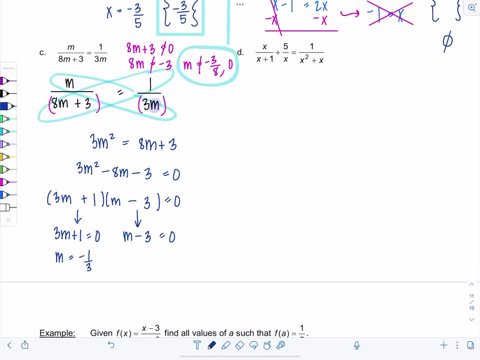 And then you're left with m equals negative 1 third or m equals 3.. Now were either one of those restrictions No, So that means both of them can go in the solution set Negative 1 third as well as 3.. 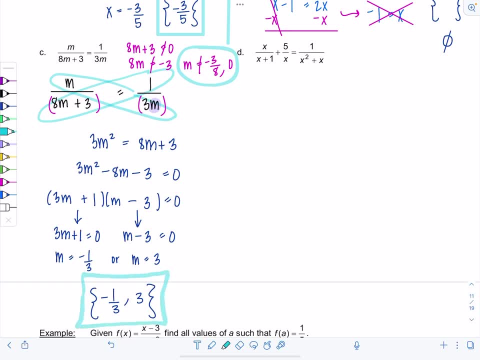 So sometimes you come out rather victorious. Look at us with two solutions this time, So fancy Making up for having Having no solution on the last one. Okay, Example D: We've got x over x plus 1 plus 5 over x equals 1 over x squared plus x. 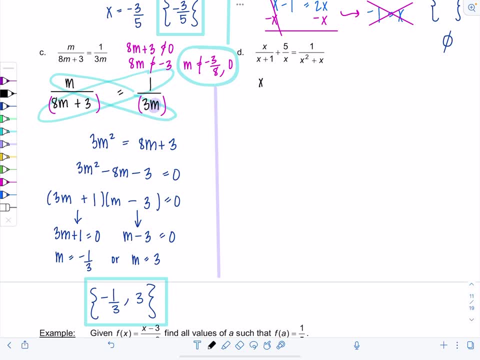 So let's start off, factor all our denominators, So we've got x over x plus 1, that's factored plus 5 over x equals 1.. And then over now, how do you factor that denominator there? Very good, 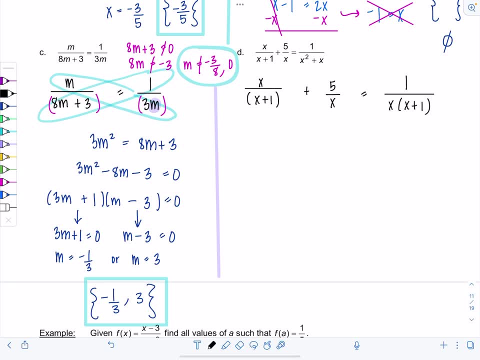 Just take out an x times x plus 1.. Okay so let's list our restrictions. X cannot equal well, negative 1 or 0, right, Which are repeated over here. So negative 1 or 0. Good, good. 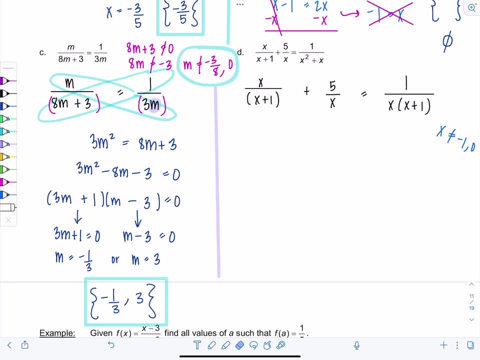 And then let's see What's the LCD. Okay, Let's see What is that LCD. Well, it needs to, for sure, include x plus 1 and x, and then those are both taken care of here. So I'm going to multiply the entire equation by x and x plus 1.. 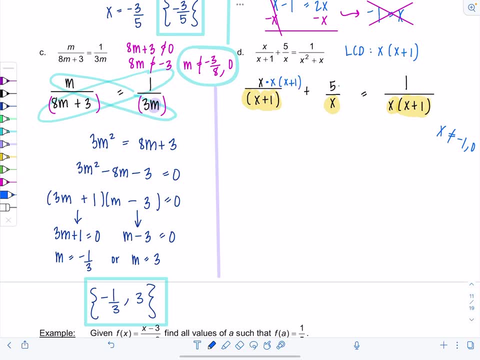 Always in the numerator: x x plus 1, x x plus 1, x x plus 1.. Don't get a common denominator. Your goal is to clear out the denominators. I see students do that over and over. 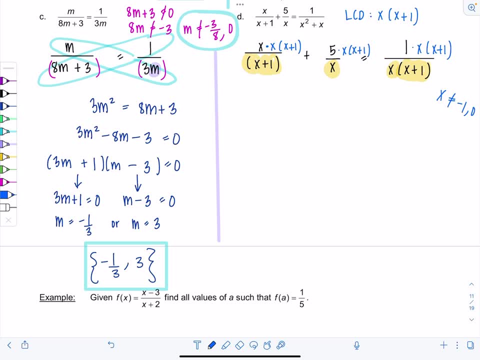 I think because you get so good at adding from the previous lesson, you get too excited. Okay, Let's cancel out. X plus 1, gone. This first term now becomes cute little x squared. How harmless. Plus x cancels. 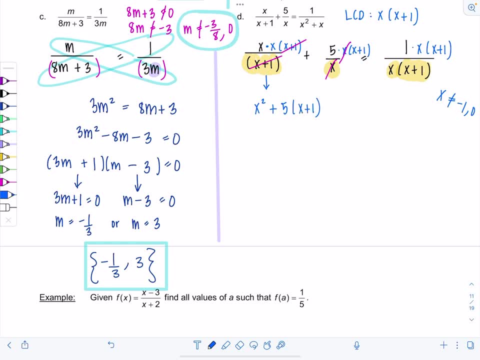 So I've got 5 times x plus 1.. Okay, So now you have x plus 1.. And then what about on the right-hand side? X cancels, so does x plus 1. And all I'm left with is 1.. 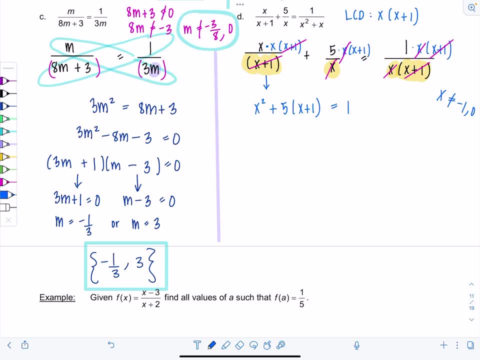 Okay, good, Aren't things looking better already? I'm telling you: Okay, So let's distribute that 5.. X squared plus 5x plus 5 equals 1. Anytime you see that you've got x squared in your equation, you have a quadratic equation. 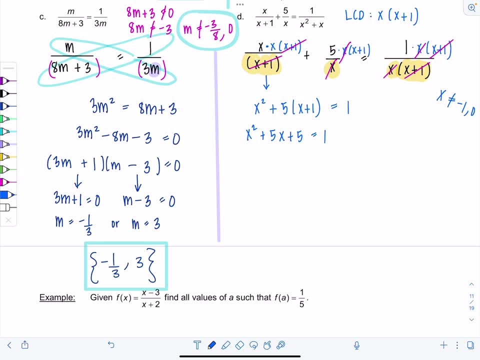 you get x squared in your equation. It's just one. Okay, All right, Let's do it again. Okay, Okay, Okay. equation: set it equal to 0.. That's the best way to go. So x squared plus 5x plus 4 is 0.. 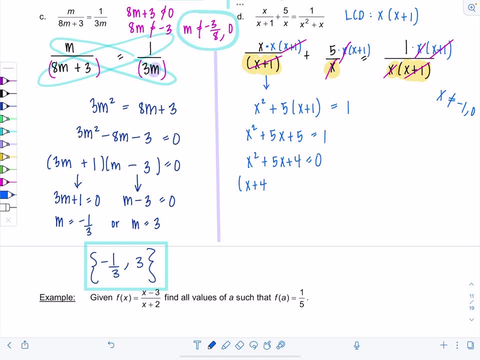 And then we can factor x plus 4 times: x plus 1 is 0. So our two solutions are going to be: can you just set them equal to 0 in your head? Oh good, So x equals negative 4 or x equals. 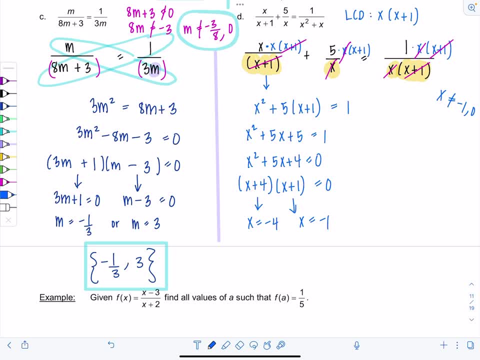 negative 1.. All right, so let's put them in our solution set. Are they both allowed in? No, they are not. Remember our restrictions were negative 1 and 0, so we can't put negative 1 in the solution set, But you can put negative 4.. Okay, so that's a big reason why I do tell my 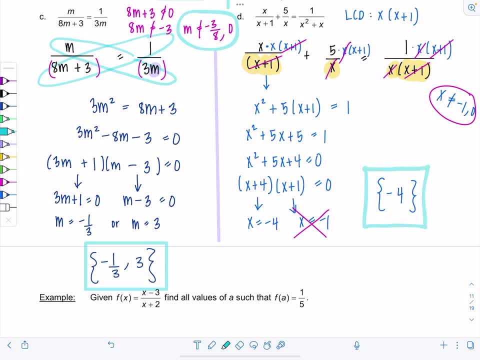 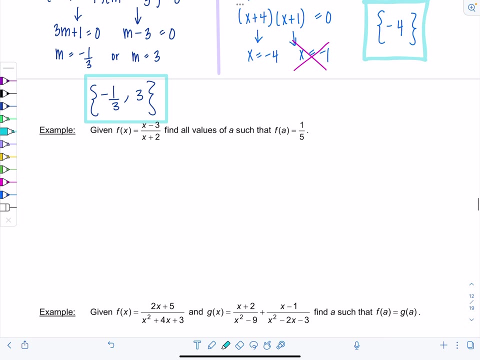 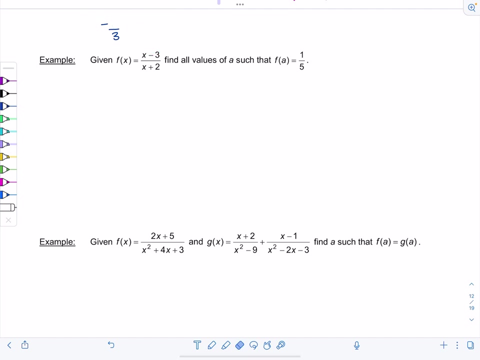 students to put a solution set every time they solve an equation, because it will remind you to take that extra step to check that you're not accidentally including any restricted values in your final answer. Okay, Very good, Let's move on. Given that f of x equals x minus 3 over x plus 2,. 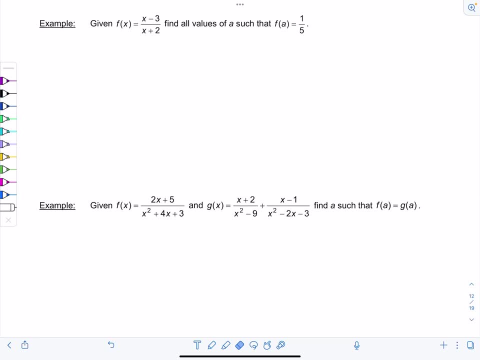 find all values of a such that f of a equals one fifth. Okay, so let's just- you know, a lot of your success in math depends on being obedient and following directions. Find all values of a such that f of a equal to 1- 5th. That's all we got to do. So f of a means: replace x with a Yep, a minus 3 over a. 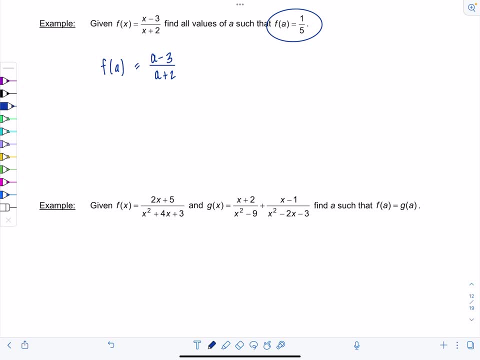 plus 2.. And they want us to find all values of a such that f of a equals 1, 5th right. So set the function equal to 1, 5th after swapping out all the x's for a's. Why? Because they told us to. 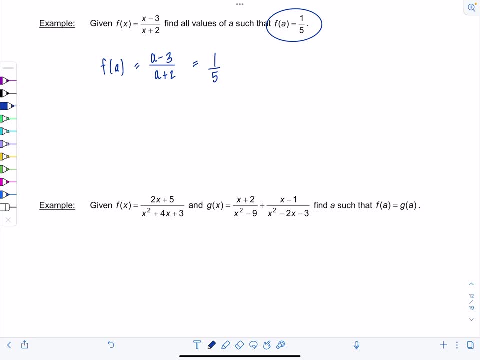 okay, The less you question in your initial math career, the better it'll go for you. Okay, let's list our restrictions. This part, basically, is the equation that we're focusing on right here. Notice we have a plus 2 in the denominator, So that means a cannot equal negative. 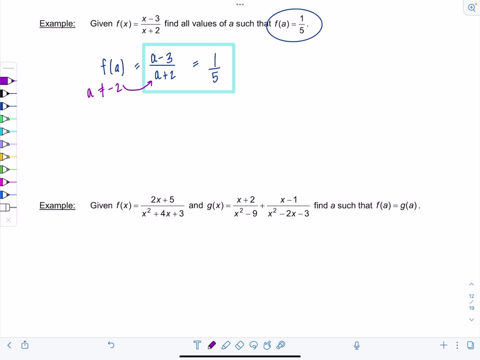 2. I'm not worried about the 5 because that's a constant. all right, You can multiply both sides by the LCD. Do you remember a little shortcut we just did a few examples ago? Yes, we cross multiplied, Wasn't it exhilarating? You can set one diagonal product equal to the 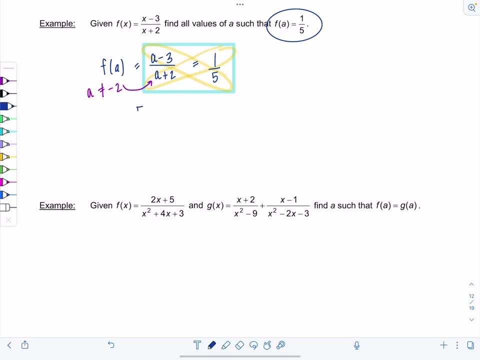 other. So let's just do it again: 5 times a minus 3 equals 1 times a plus 2.. Love it. So let's distribute: 5a minus 15 equals a plus 2.. I'm noticing, oh, there's no squared terms, right? So 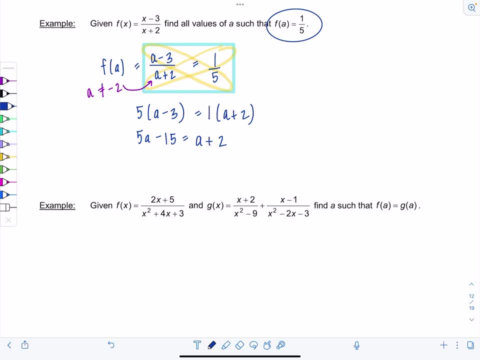 I'm not going to set this equal to zero, I'm just going to put all the variables on one side, all the constants on the other. So, subtracting a from both sides, we've got 4a. add 15 over equals 17. So a equals 17 over 4.. Okay, that wasn't one of our restrictions, So we're good. 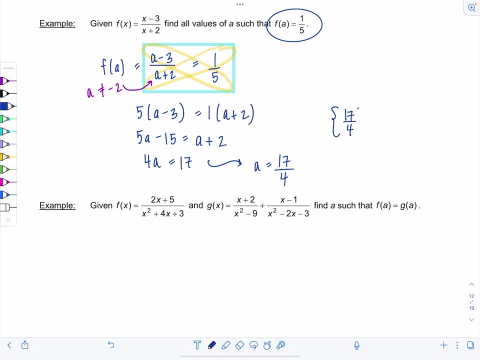 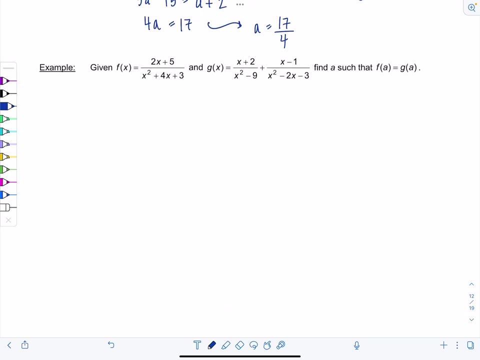 You can put a solution set if you want. We answered the question. okay. Very nice, I got one more for you. Are you ready? Good. So, given f of x equals 2x plus 5 over x squared plus 4x plus 3, and g of x equals x plus 2 over x squared minus 9 plus x minus 1 over x. 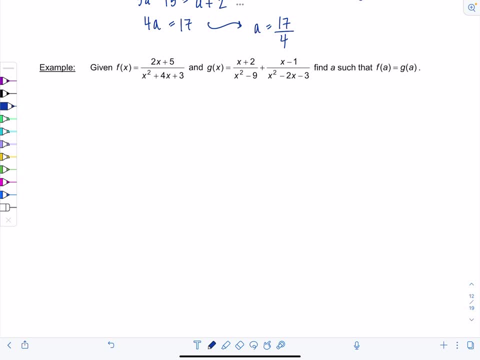 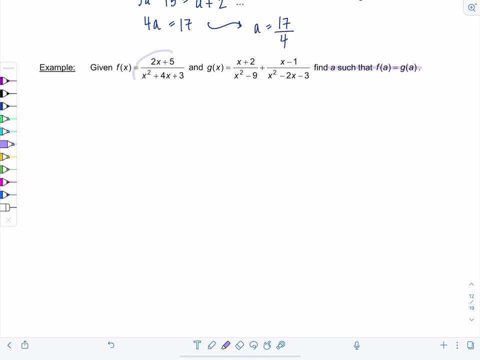 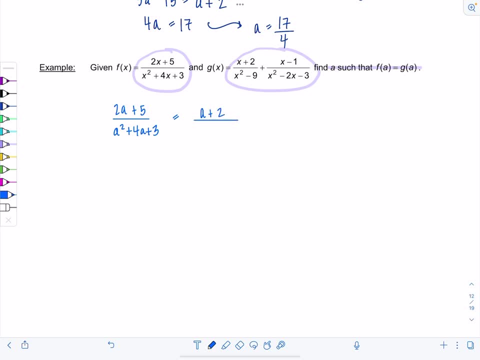 We're going to set that equal to A plus 2 over A squared minus 9 plus A minus 1. we're going to set these two functions equal to each other and solve, but also they want us to 1 over a squared minus 2a minus 3.. Very good, Okay. now let's start off following our normal. 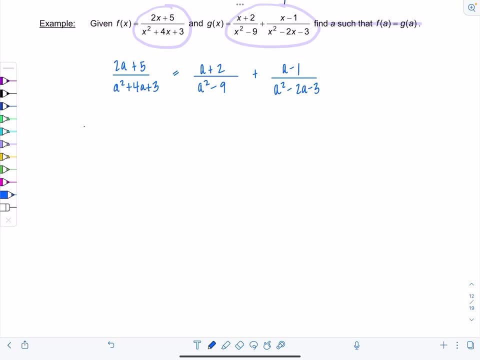 process. Factor all the denominators, just the denominators. okay, Oops, squiggly line, Straighten up, get your act together. Okay, a squared plus 4a plus 3, that's a plus 3 times a plus 1. This equals a plus 2 over. how does a squared minus 9 factor? 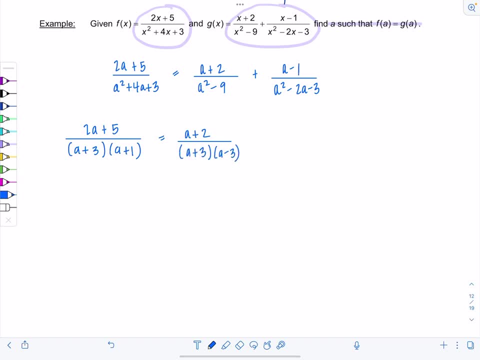 Excellent. a plus 3a minus 3, plus a minus 1. over, uh-huh, a minus 3 times a plus 1.. Very good, Let's list the restrictions, Restrictions, So a cannot equal. let's. let's see we've got negative 3, negative 1, and positive 3, right, All the others are repeats. 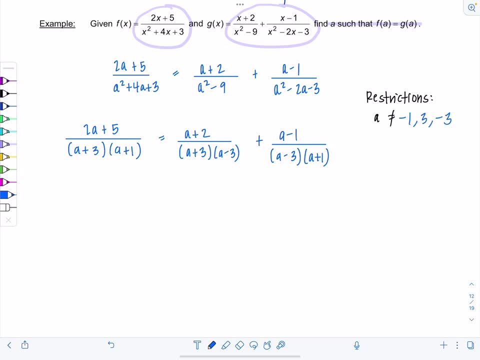 So negative 1,, positive 3, or negative 3.. Good, Save that. Did you figure out what the LCD is? So we've got a plus 3,, a plus 1, and a minus 3.. Good, Don't repeat a factor if it only appears once in each of the denominators. okay, 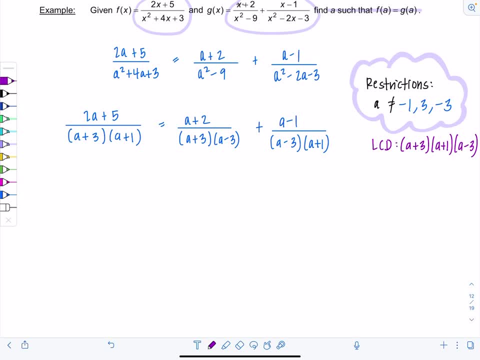 Very good, Now I multiply every single term by the LCD in the numerator upstairs. okay, So we're going to hit this with an: a plus 3, a plus 1, a minus 3.. Now I'm going to be honest. 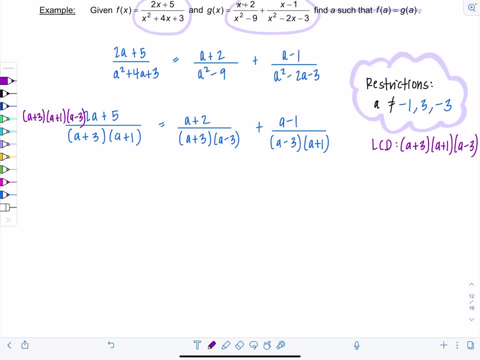 you guys, I don't normally write it next to each term, I just write it once off to the side with big old brackets. But I want you guys to really clearly see how everything cancels. so I'm not taking shortcuts, But just so you know you can just write the LCD once and then put like brackets out here. 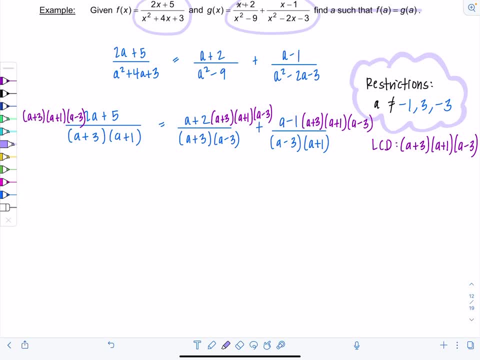 Do you know what I mean? Okay, I just didn't want to scare you all. Okay, a plus 3 is going to cancel over here. This part's always so satisfying. A plus 1, gone, And then what's left? Oh. 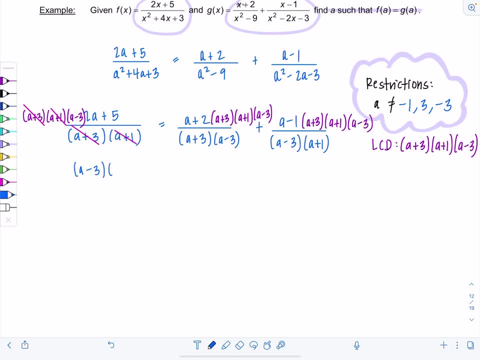 just sweet little: a minus 3 times 2a plus 5.. Okay, And then this equals- let's see what's going on over here: A plus 3 is gone, A minus 3 is gone. So what's left? A plus 2,, please put. 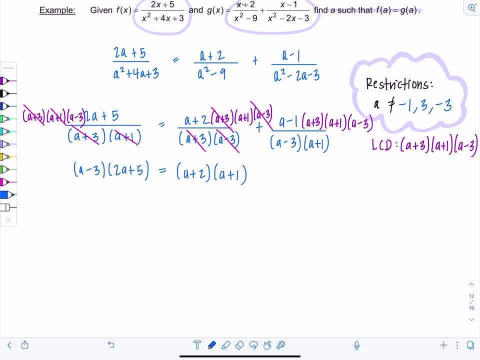 parentheses around it times a plus 1.. Plus, last term, a minus 3 is gone, A plus 1 is gone And I just have yes, yes, yes, put parentheses: a minus 1, a plus 3.. Okay, time to foil all these suckers out. 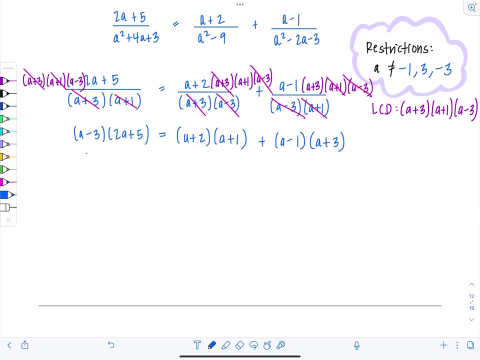 Foil party time. This is 2a squared plus 5a minus 6a minus 15, yes, And then the others. we can do quickly a squared plus 3a plus 2 plus a squared 3 minus 1, that's going to be plus. 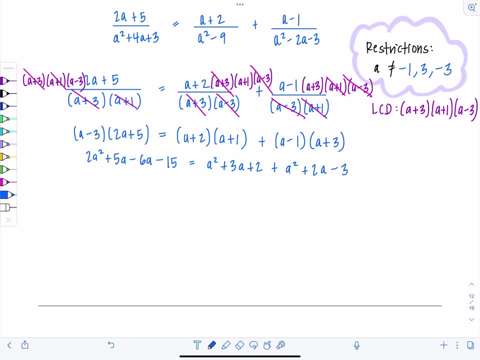 4th, a minus 3.. Okay, So we've got here 2a squared minus a minus 15, equals. I've got 2a squared also over here, right? Combine these a squares plus 5a and then 2a negative 3 is going. to give me minus 1.. Okay, times a minus 10残3, 0.88.. So again, that's going to to give 5a minus 5.. And the other 2a squared minus 15, I adopt. However, I forgot the numbers. I'm going. to excuse my favorites, So I just kinda avoid them. Okay, Coin a squared by two minus a shoulder, 2a minus three. Okay, So we've got here 2a squared minus a minus 15, equals. I've got 2a squared also over. 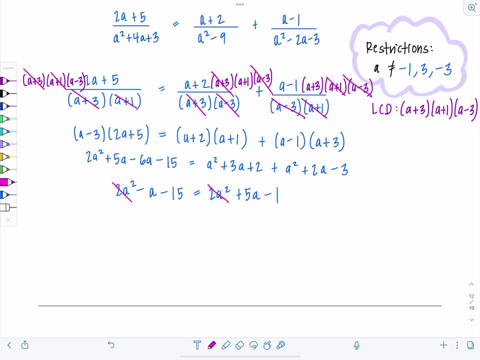 here, right, Combine these little a squares plus 5 a, and then 2a negative 3 is going to give me minus 1. squared cancels from both sides. Oh wow, So we no longer have a quadratic equation. I'm going to. 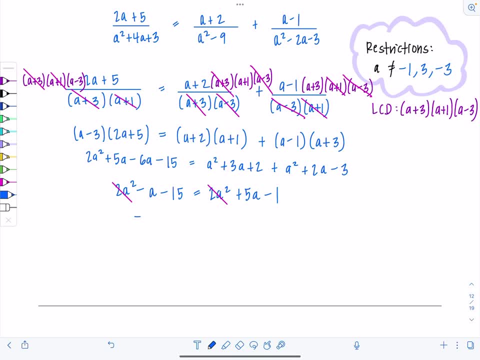 put all the a's on the left. So subtract 5a from both sides, That's minus 6a. minus 15 equals negative 1. Add 15.. Negative 6a equals positive 14. So a equals negative 14 over 6. Always put. 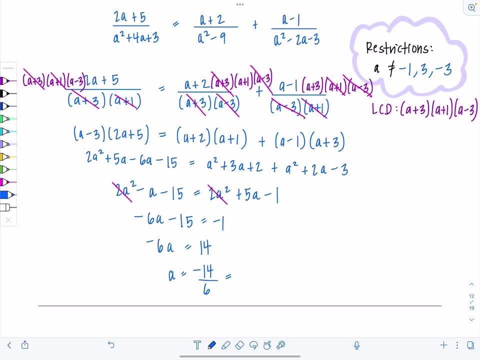 your negatives in the numerator, you guys, And that reduces to negative 7 over 3.. Was that one of our restrictions? No, So we can put it in the solution set with a clean conscience. I always feel defeated at the end. you know when I have no solution. 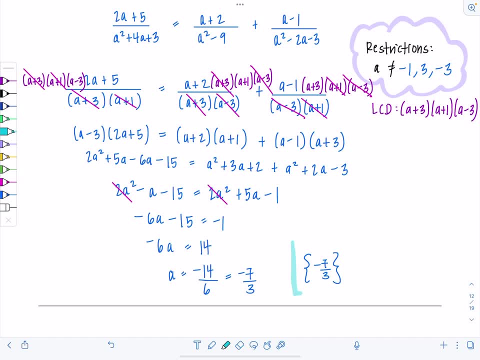 Not that it's any fault on my part, but I like to report an answer. Do you feel the same way? Comment below. Let me know if you get a little sad when you get no solution, or is it just me? So that concludes the video. If you found it helpful, please give it a thumbs up. Subscribe. 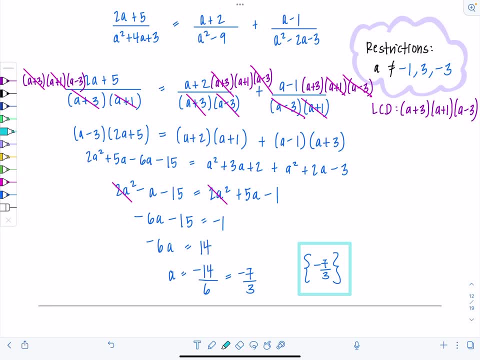 if you haven't already, Really helps my channel. pop up more and be able to help more students around the world, which is my goal. So stay tuned. We've got solving applications, aka word problems, using rational equations and other algebra topics your way. 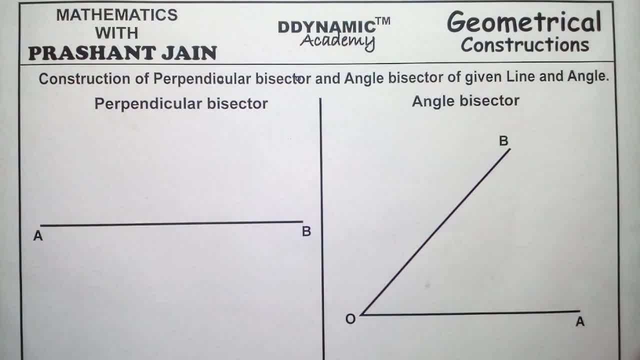 Good morning viewers. How are you? Hopefully all of you are healthy and fit Myself, Prashant Jain. This time I am with the videos of some geometrical constructions And the problem this time: how to draw a perpendicular bisector on a given line segment. 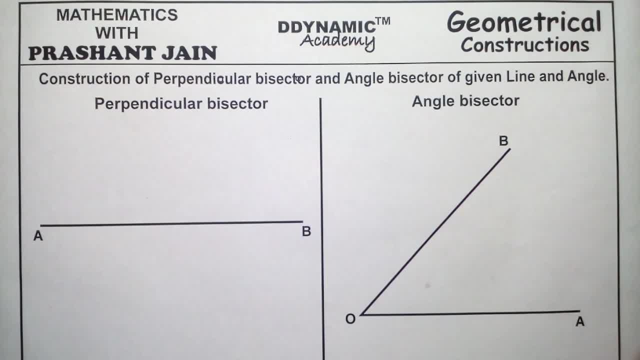 The meaning of the perpendicular bisector is to construct a line in such a way that divides a line segment into two parts, such that it makes an angle of 90 degree with the given line segment. In front of you, you see that there is a line segment A, B, I don't know how much the length of this line segment. Now we have to detraw the perpendicular bisector of this line segment.